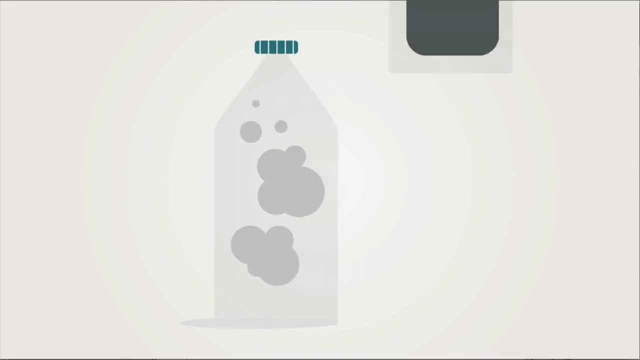 and squash them into a bottle so that they can be weighed. compared with the weight of petrol burnt, the exhaust gases will weigh much heavier because oxygen from the air has been added. Here is a bit of a petrol molecule: H2CCH2.. It joins with 6 oxygen atoms, or 3. 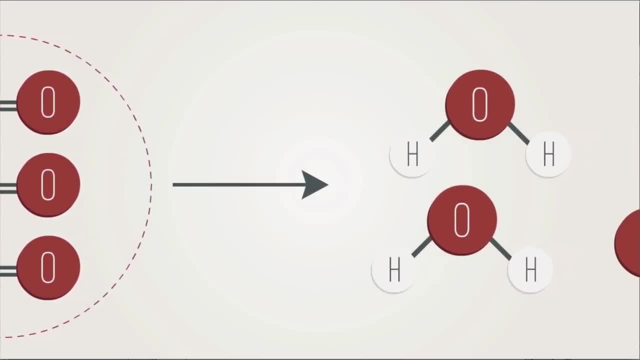 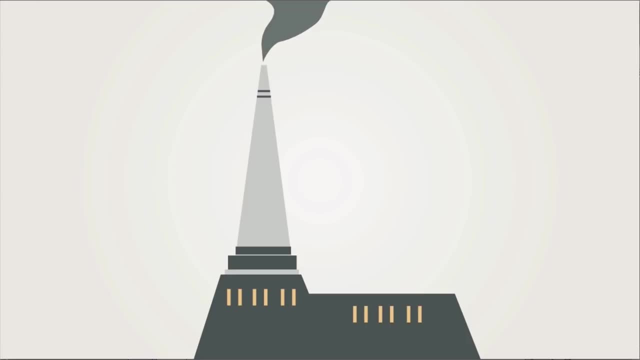 molecules to build up: hydrogen oxide or water vapour, and carbon dioxide, another two molecules. Before the world became industrialised by burning fossil fuels, the carbon dioxide concentration in the atmosphere was about 0.28%- tiny compared with oxygen at 21% and nitrogen at 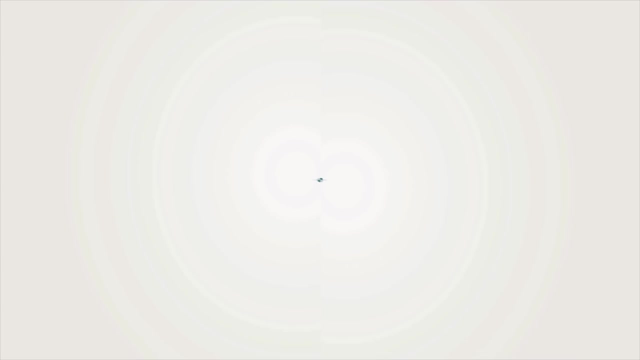 78%, but enough to keep us warm. Without this natural blanket of insulating gas, the earth would be too cold to support life as we know it. But this carbon dioxide released when fossil fuels burn adds to the existing carbon dioxide levels, which are now nearly 50% higher. 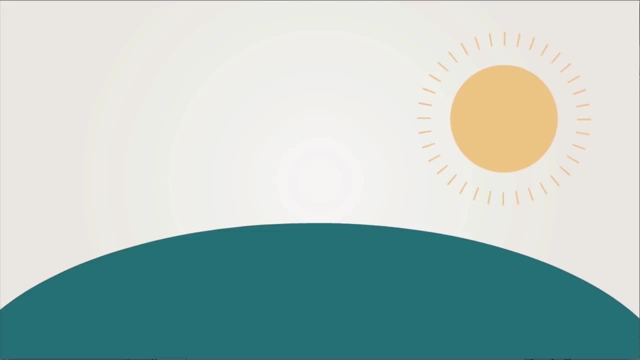 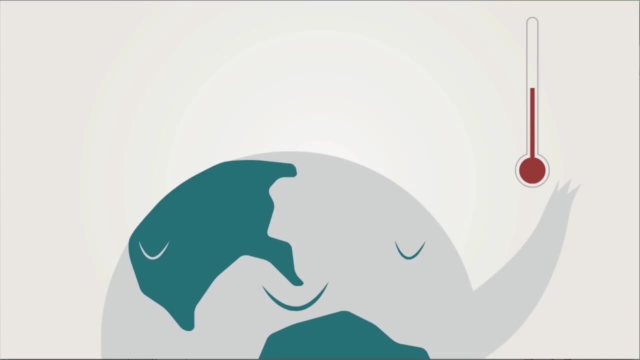 than in pre-industrial times. Although we get a daily supply of heat from the sun, the earth normally loses this at night and in the cooler seasons, so that the average temperature of the earth remains constant, But this status quo is starting to change, As humanity adds. 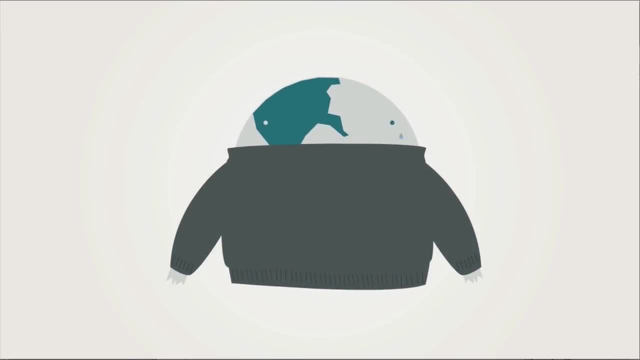 carbon dioxide into our atmosphere. it is as if we are putting a sweater round the planet. The extra layer isolates the heat and it cannot escape as easily. Whilst it is easy to take off your sweater, it is not as easy to take off your sweater as it is to take off your. 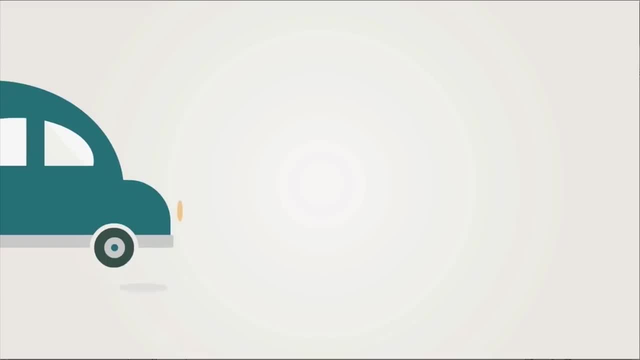 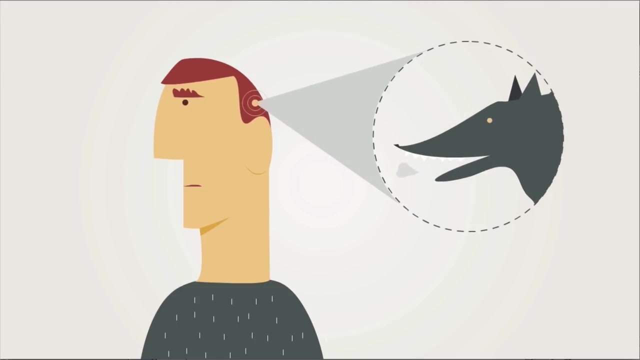 sweater. The earth cannot lose it greenhouse gases as quickly and we keep adding to them. By putting our planet in a sweat box, we are causing wide-ranging consequences for our climate. Some people think that living things contribute to the enhanced greenhouse effect because they breathe out carbon dioxide, but this carbon has come from their food and 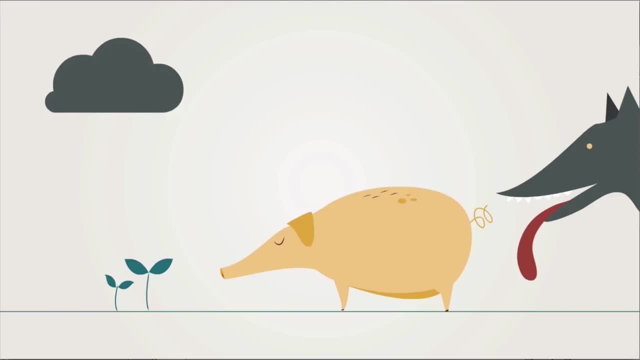 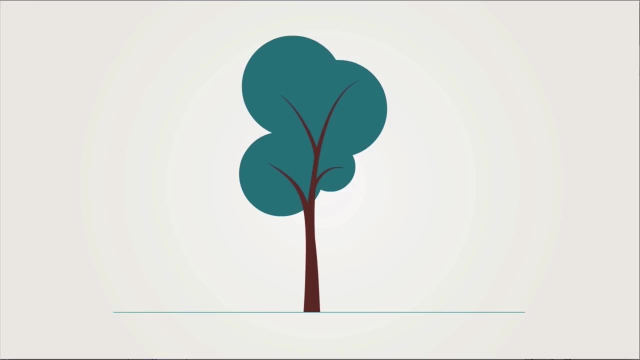 that's come from plants which took carbon from the atmosphere in what is called the Carbon Cycle. There's a video for that. Even burning wood doesn't contribute to the enhanced greenhouse effect, as long as the trees you cut down are replanted. However, the carbon in fossil fuels has remained trapped underground for